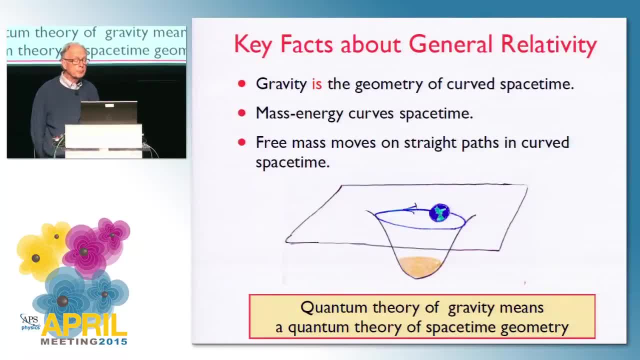 That's the classical theory, But it has important implications for the quantum theory because it means that if you're going to construct a quantum theory, it's a quantum theory of gravity, It's a quantum theory of space-time geometry that will assign probabilities to different space-time geometries. 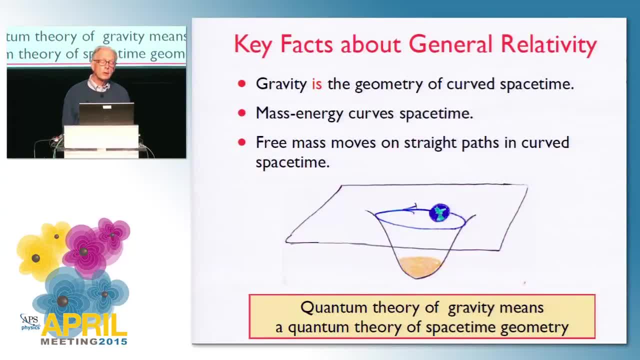 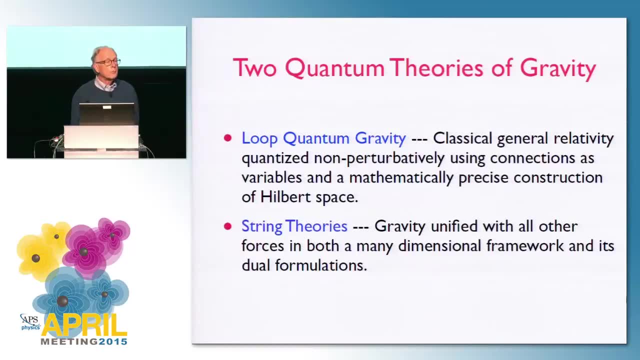 what their configurations are given a quantum state. Right now there are, at least right, two big theories of quantum gravity. There's loop quantum gravity, which is a theory of quantum gravity which is a non-perturbative effort to quantize classical general relativity. 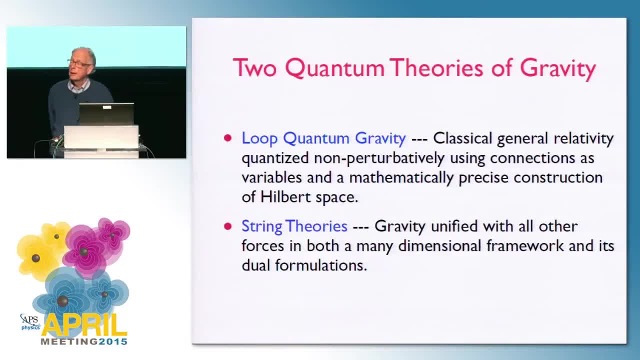 using connections as variables and a mathematically precise construction of Hilbert space, And it's advanced quite far and has many predictions. There's also string theories, gravity unified with other forces in an essential way to make sense out of gravity in a multidimensional framework. 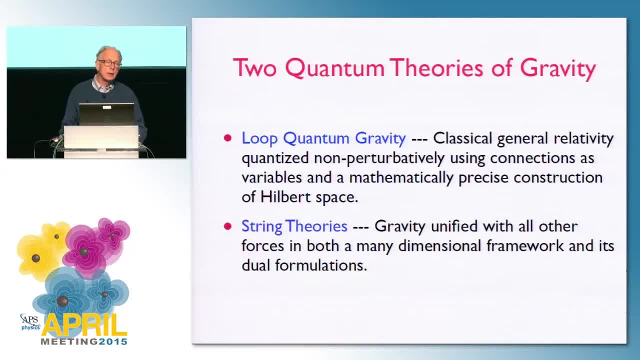 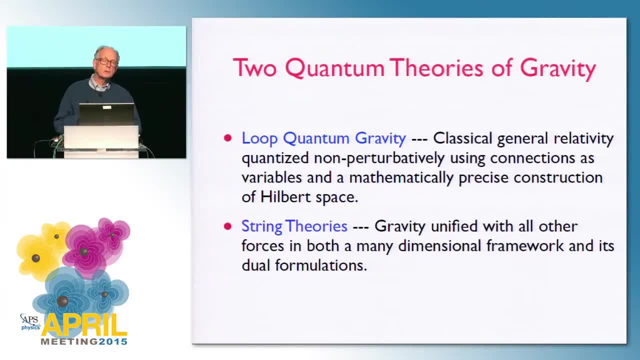 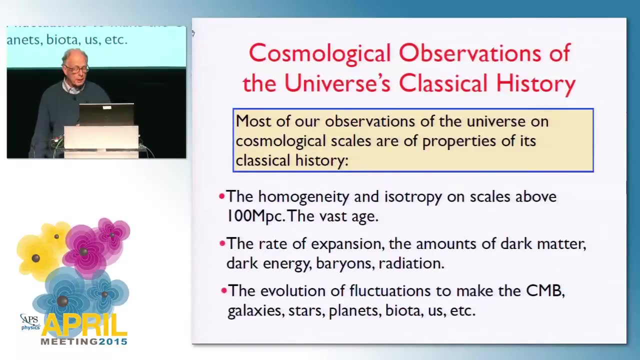 My understanding of the organizers is they would. from the organizers is that they would like a review of these two theories in a half an hour. That's not going to be possible, So instead I'm going to address the question of why are we doing this at all? 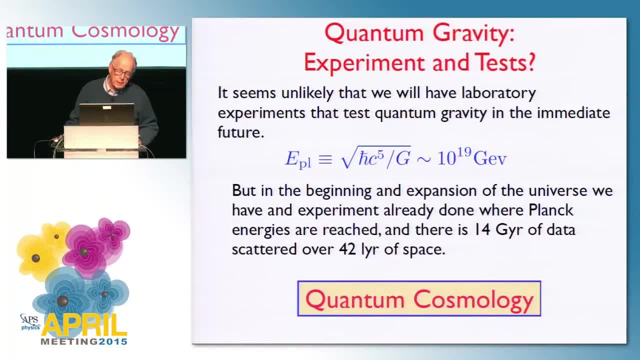 What are their predictions? What are the outcomes? It seems unlikely that we're going to have a laboratory experiments that test any theory of quantum gravity in the immediate future. The scales, the natural scale, the Planck scale constructed from H, bars C and G, is way too high. 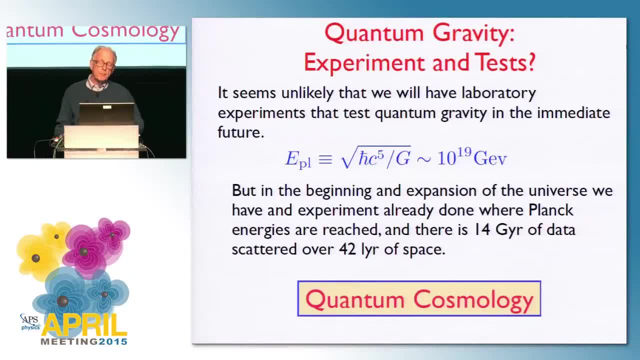 People argue over whether the scale be lower by modifying their theory, but we still have to face that dimensional number. So we are unlikely to have laboratory experiments. but we have one big experiment that we're in the middle of, In the beginning, in the expansion of the universe. 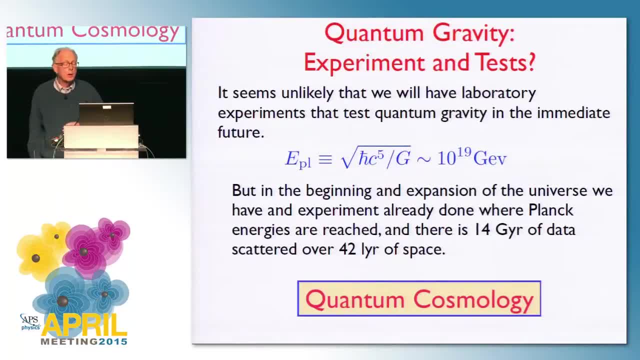 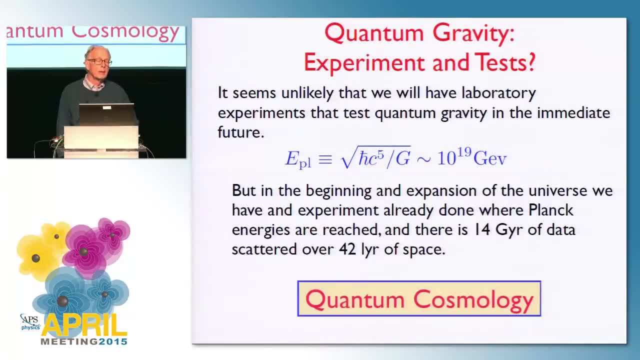 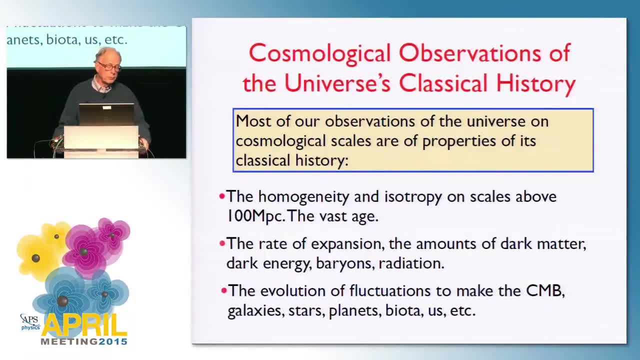 Right, Right, Right, Right, Right, Right, Right. I mentioned that the theory of quantum gravity would predict probabilities for different space times. Most of our observations of the universe on cosmological scales, or at least some of them right, are properties of its classical history. 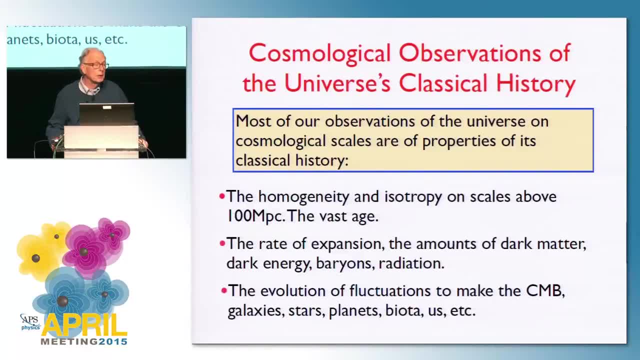 The homogeneity and isotropy we see on scales above 100 megaparsecs, The vast age of the universe, at least when measured in Planck units, order 10 to the 60th Expansion seen in the Hubble constant, the amounts of dark matter, dark energy, baryons. 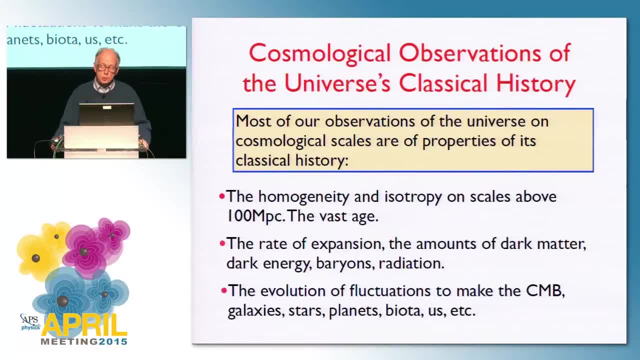 and radiation- all relics from a very early stage, And the evolution within the universe of quantum mechanical systems to make the CMB described in the previous talk: galaxies, stars, planets, biota and even us. But classical behavior is not guaranteed in quantum mechanics. 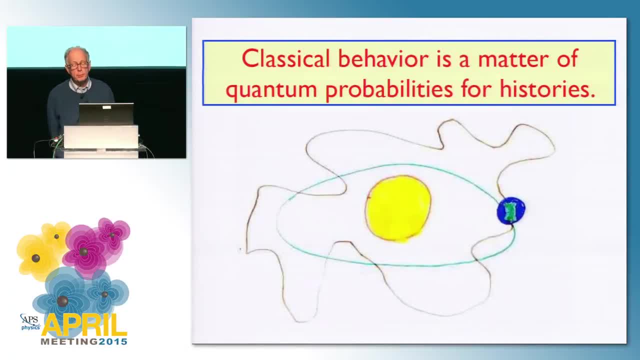 If, for example, you consider the orbit of the Earth around the sun according to quantum mechanics, there's a probability that it would take any possible orbit. It's only in the particular state that the system is in and the particular course: graining. 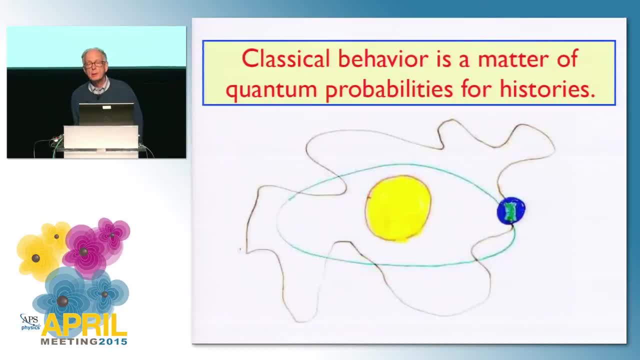 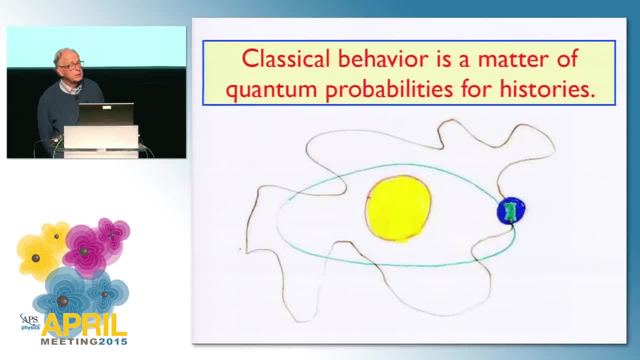 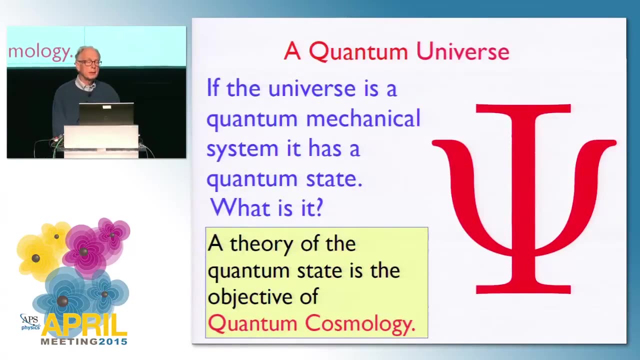 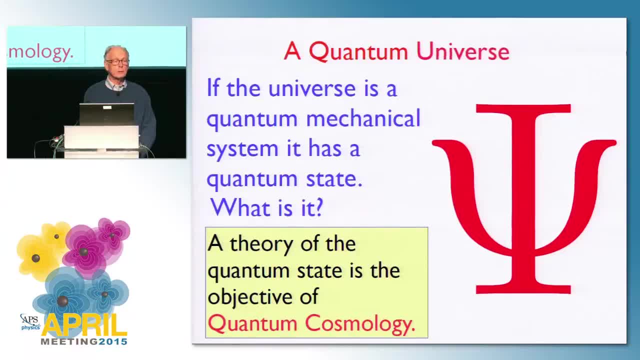 like general relativity or a string theory or even loop quantum gravity, You also need a quantum state because in quantum mechanics the probabilities are basically the squares of operators applied to the quantum state. And, of course, if we think, as we're assuming here, that the universe is a quantum mechanical system, 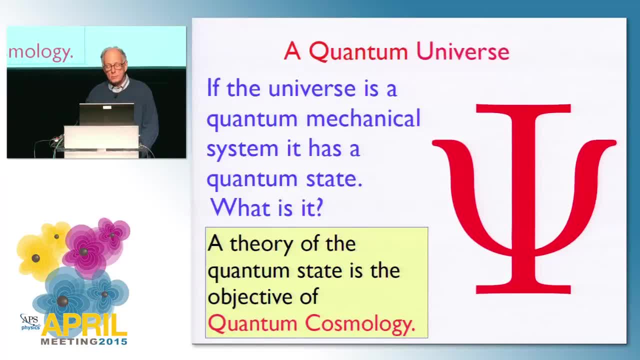 then it has a quantum state. The question is, what is it? So a theory of the quantum state is an objective of quantum cosmology. The quantum state is not something we're going to measure. our measurements are too puny to do that, and we've only got one system. 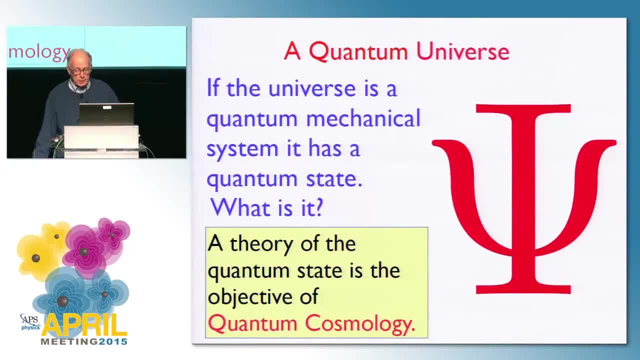 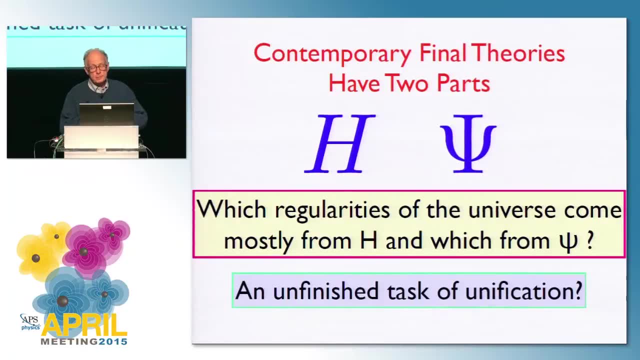 So a theory of the quantum state is in fact a necessary part of any final theory, in addition to a theory of dynamics. So it happens that contemporary final theories have two parts. They have a theory of dynamics which I've written here as H for Hamiltonian. 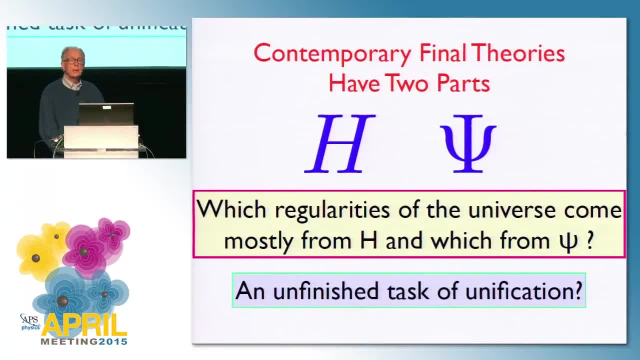 and a theory of the state. So we can ask which regularities of the universe that we see come mostly from H and mostly from the state. We can also ask a little bit later on whether there's an unfinished task of unification here to provide one theory. 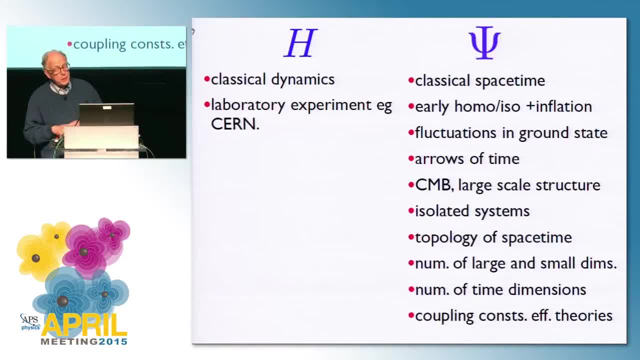 from which both would emerge. So here's a little list of regularities that we might expect in our universe, that we might expect to emerge mostly from H and mostly from the wave function. Of course they all emerge from the combination. I'm just asking which is the most important. 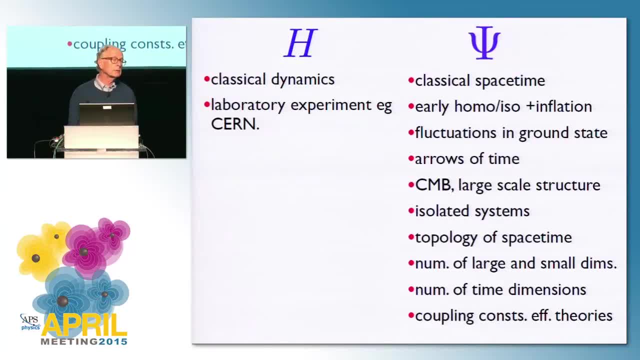 So, certainly from the Hamiltonian, we get classical dynamics, so the Einstein equations, for example, and we get predictions for laboratory experiments which are designed to be as independent as possible of any initial condition of the universe, for example at CERN. 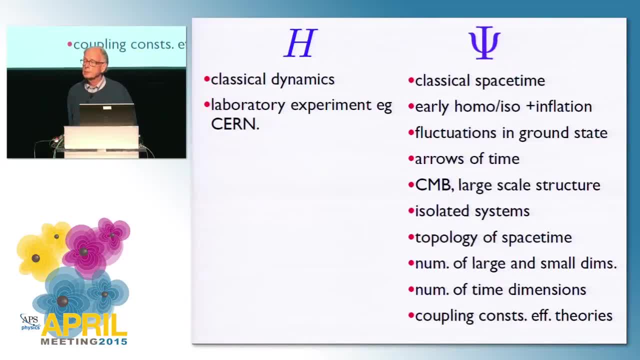 But if we look on the larger scales, most of the regularities that we see probably follow mostly from the state First, the existence of classical space-time at all, as I have described on the previous stage, and the existence, the wide range of application. 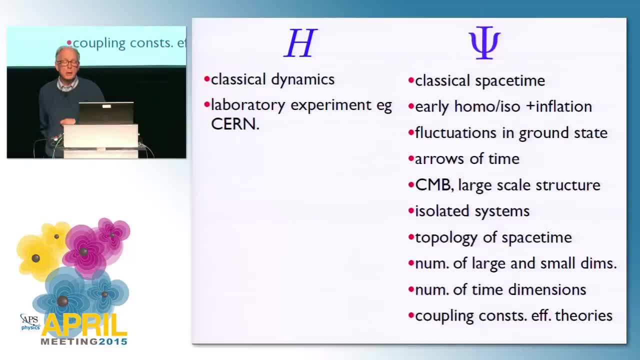 of classical physics over, as far as we can tell, the entire visible horizon on certain scales, from a short time after the Big Bang to the infinite future. Then the particular properties of the state, The early homogeneity and isotropy, now on scales above 100 megaparsecs, and so Inflation. 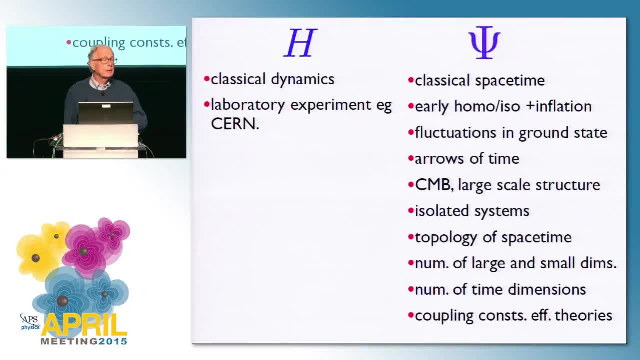 if there was, And the fluctuations away from these symmetries that we see in the CMB today and in large-scale structure of the galaxies later on in the universe Arrows of time, if the theory, if the dynamical theory, is time-reversal, invariant, as all our best candidates are. 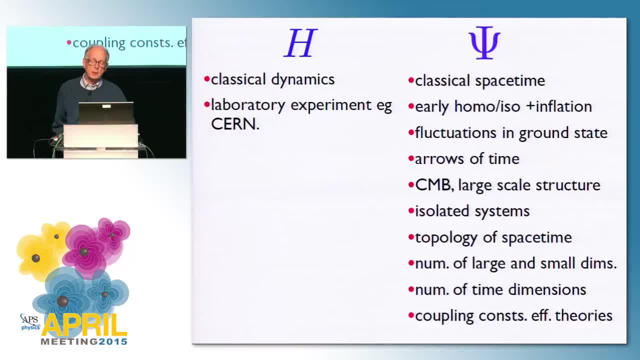 then, to explain the arrow of time, you have to say something about the quantum state, The CMB, the large-scale structure. I've already mentioned the existence of isolated systems. We're all semi-isolated systems in this room- but that's not guaranteed in the theory in any sense. 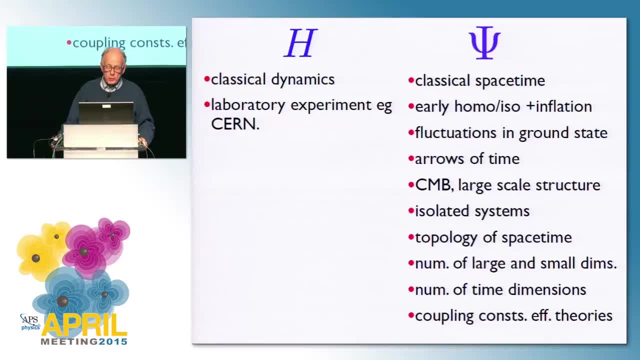 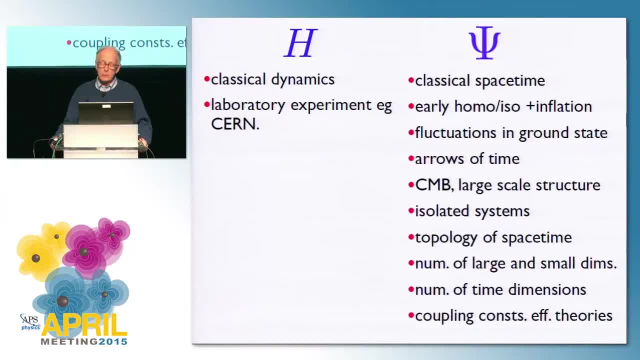 right, Whether it might be, for example, something like a Torus or a hall of mirrors or something like that, or an iris sphere, the number of large and small dimensions and the theory that has of those, the number of time dimensions, for example, coupling constants of effective. 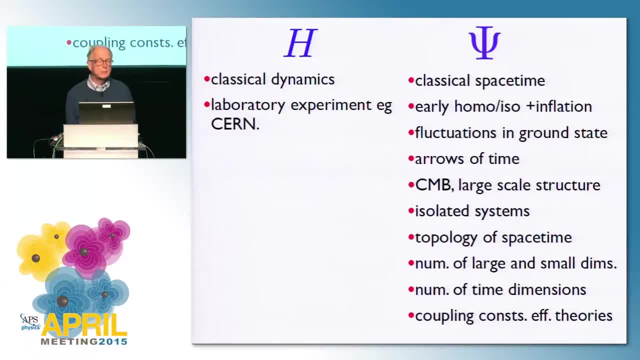 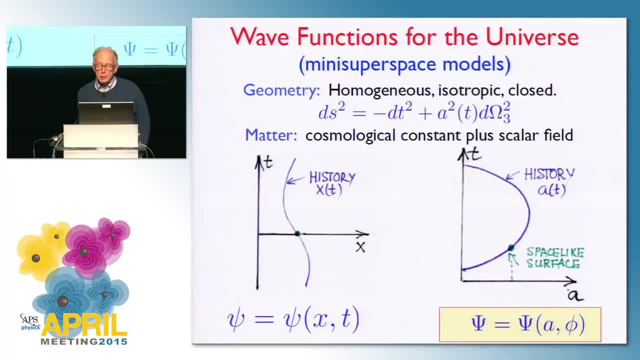 theories was a huge list of things We might hope to get out of the state. I'm going to record very briefly about those. So to do that, I'm going to give you a very quick introduction to wave functions of the universe, which represent quantum states in a very 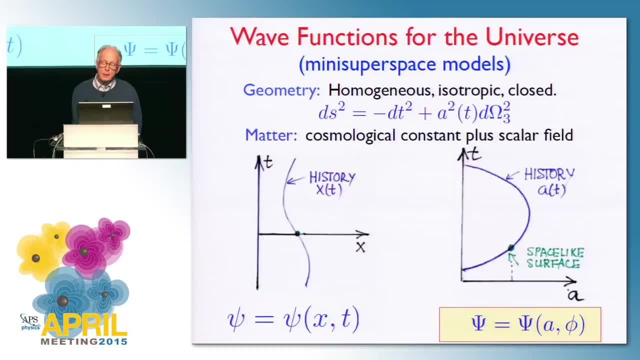 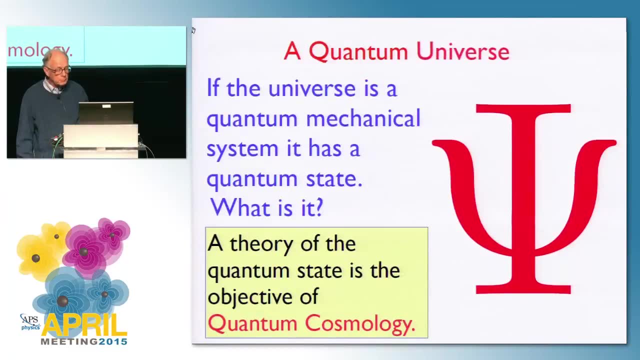 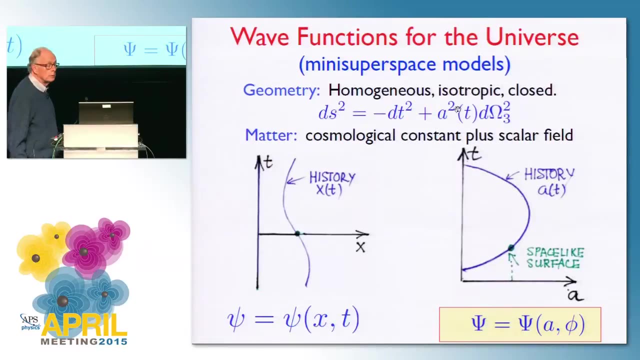 simple class of models, models which are homogeneous and isotropic and therefore have whoops. there we go all right. therefore have only one quantity, which is other, like spheres, and a, for example, is a scale factor that represents the overall size of the universe at any one time. now, in ordinary quantum mechanics wave. 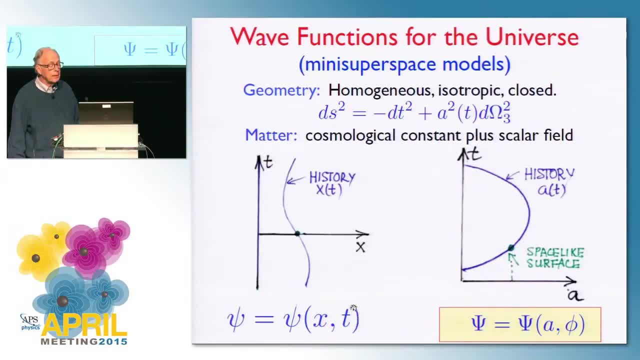 functions are functions of X and T and you can think of those as the quantities. if you have a history X of T, they tell you what they specify the history at one on one space-like surface in quantum gravity. we also have histories. here's a, for example, a history of the expansion of expanding and collapsing universe. 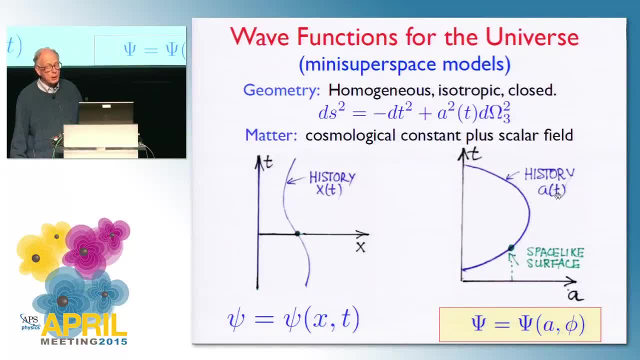 described by the scale factor a, which is a function of time. and if we have a scalar field in addition to the geometry, it's usually argued that the wave. you don't need an additional time variable right to label what points you are, because the size of the universe itself tells you where you are in this curve. so 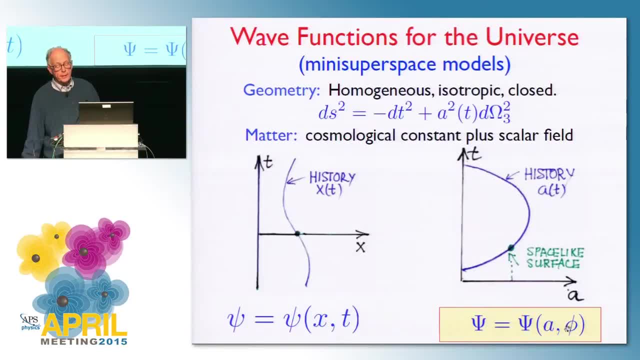 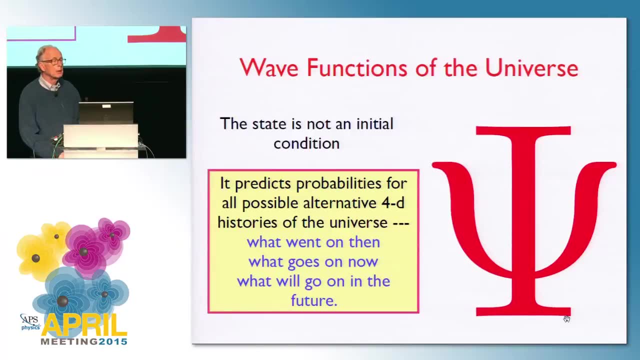 wave functions, in a very simple model, would be a function of scale factor and one field, let's say, for example, scalar field. it's important to stress that wave functions of the universe are not an initial condition, because initial and final already presumed that you have a notion of space-time and we're seeking 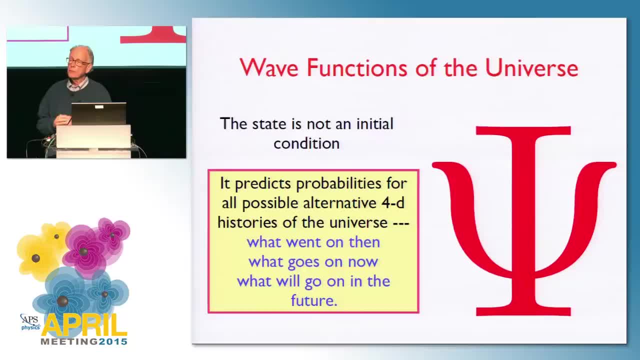 to produce the notion of classical space-time, so you have to think of them in four-dimensional senses, as representing something that will tell you what went on in a four-dimensional way, what went on then, what goes on now and what will go on in the future, and that way it becomes predictive. now I'm going. 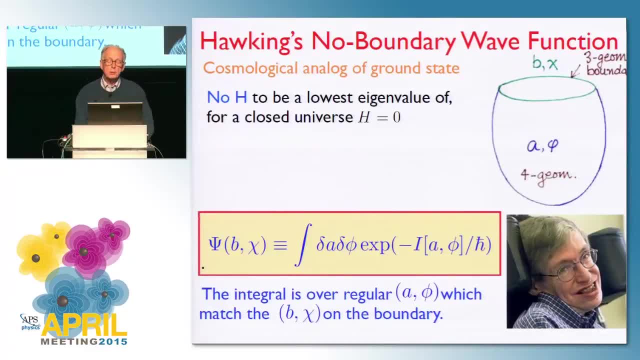 to report on one particular state right, which is Hawking's no boundary, of the wave function of the universe only because that's been the most developed. this wave function is the analog for closed cosmologies right of the ground state, an ordinary field theory, and since there's plenty of 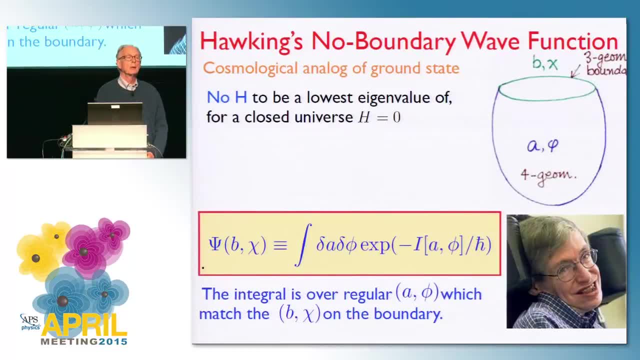 evidence. the ground states typically are very simple and the early universe was very simple, more homogeneous, more isotropic, more nearly in thermal equilibrium. that that might be a good candidate for the quantum state, theoretically based on a rough connection with observations. but you can't in a closed cosmology. 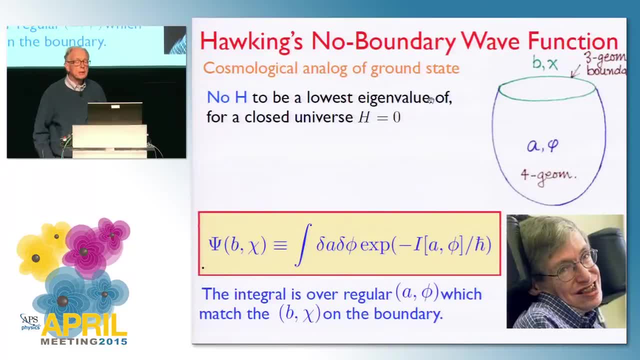 think of a ground state as being the lowest eigenfunction of some Hamiltonian, because from the diffeomorphism and variance of general relativity the closed cosmology of the Hamiltonian vanishes identically. Also, everything is an eigenstate of it. 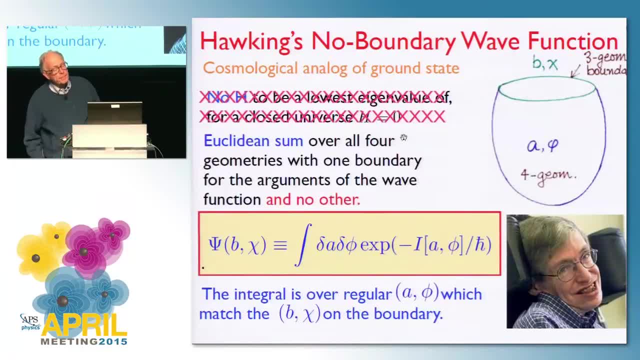 But in ordinary field theory there is another way of constructing the bound state: by a Euclidean sum over all histories that match the arguments of the wave function, And so we can construct a state which is the Euclidean sum over all four-dimensional geometries. 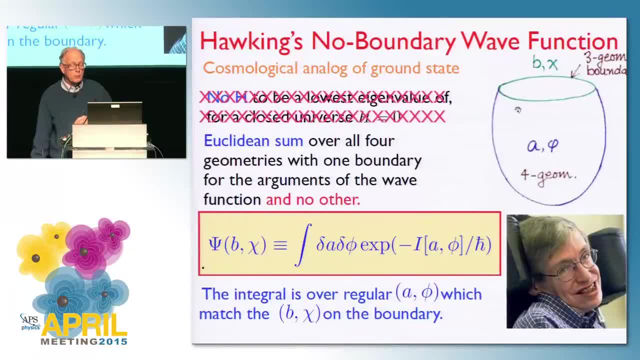 that have one boundary right where the arguments of the wave function. this is supposed to be a four-dimensional geometry scale factor, four-dimensional scalar field matching a three-geometry and a three-dimensional scalar field, and we just do an integral. 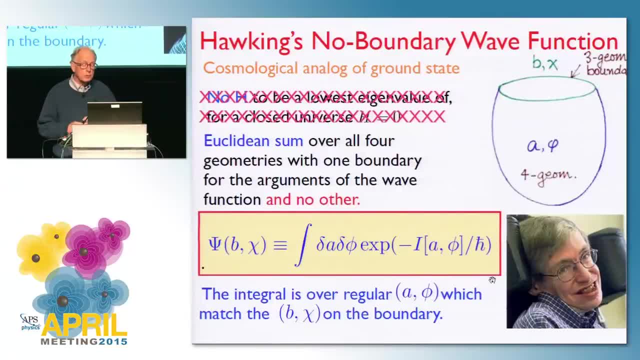 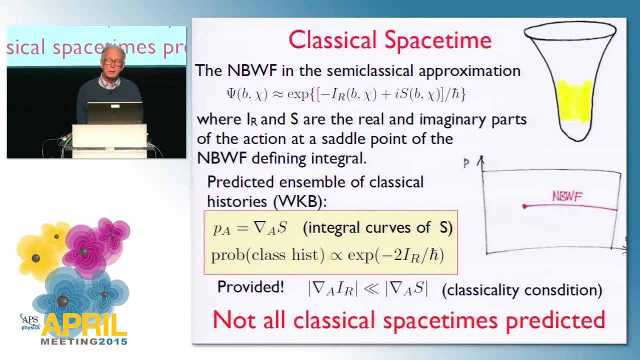 over e to the minus the action of the theory, and we produce a wave function which is the analog of the ground state and that is the candidate I'll discuss for a wave function of the universe. So, first of all, how do we predict that there's any classical spacetime at all? 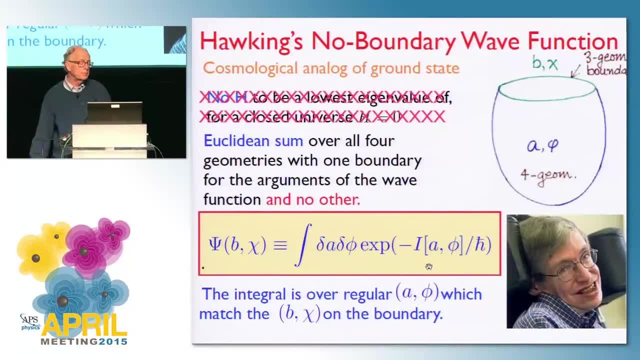 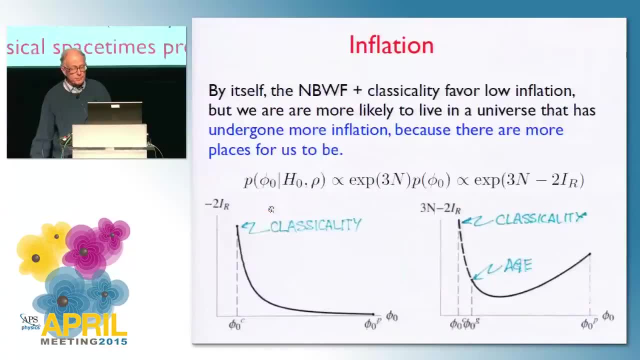 This integral which I showed you in the previous slide. imagine it doing my steepest ascents, Then you, basically the result will get e to the minus times, the extrema of the action and the no-boundary wave function. therefore, 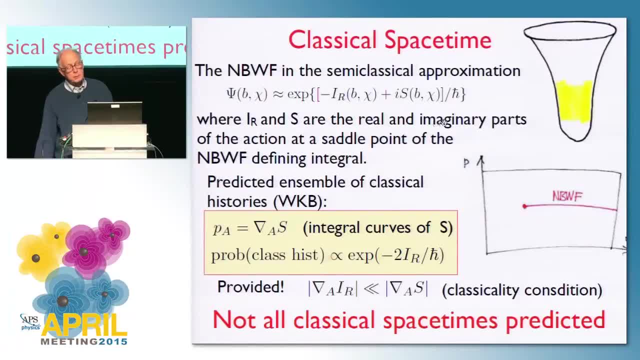 predicts something like this. Since the extrema are generally complex, I've tried to draw a picture of one here. right, Here's the one boundary where the wave function is defined and that's the no-other boundary, and this is complex. 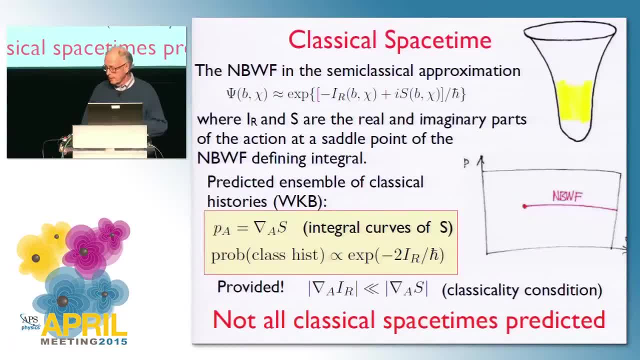 We call them fuzzy instantons, but there's no particular reason for that. At any rate, the state would have this form and it will have a real part, an imaginary part, to the action. but that should look familiar to you. It's ordinary WKB. 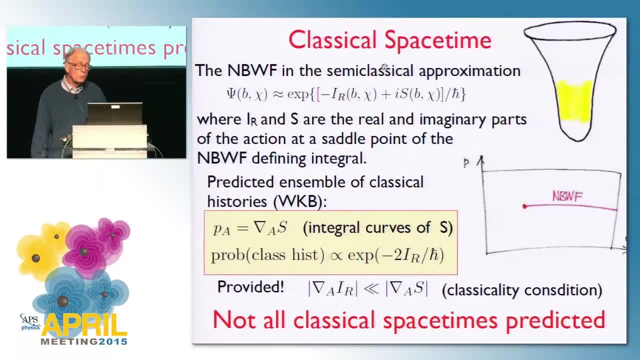 And so we predict an ensemble of classical spacetimes which are the integral curves of the imaginary part of the action here, that is, the solutions to the Hamel-Nyokomi equations. momenta equals the gradient of s, and the probability is roughly the square of the wave function. 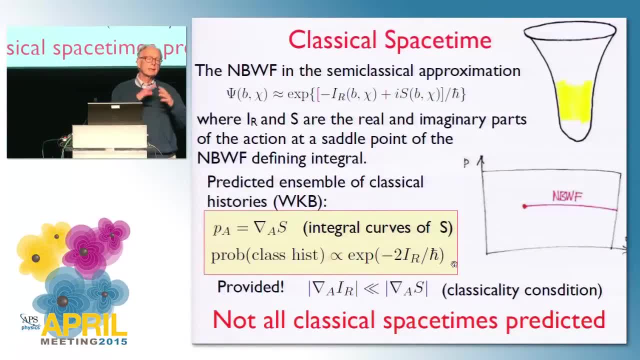 which is e to the minus 2ir. So thus we've predicted an ensemble of possible classical spacetimes for what the universe might be like, with probabilities for what they are. And not all classical spacetimes are predicted. Um, whoops. 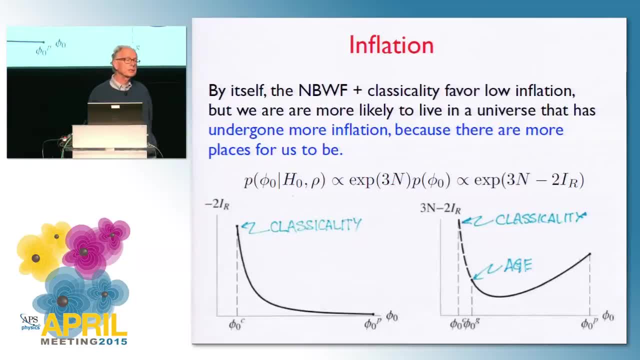 So let's just give one simple example. Ask the question: um does the no-boundary predict wave function predict the high probabilities for inflation in the early universe? The answer is no. it does not By itself. it predicts all that. all early histories inflate. 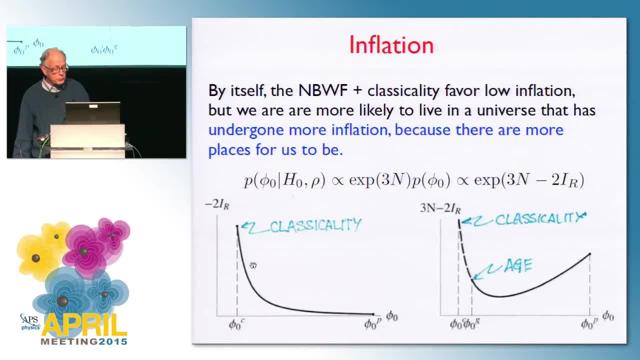 but the probability for inflation, for the number of e-folds, roughly here uh, is um declining. But in cosmology you have to take into effect that everything is inside, including us, as observers uh, which are also quantum mechanical systems in the universe. 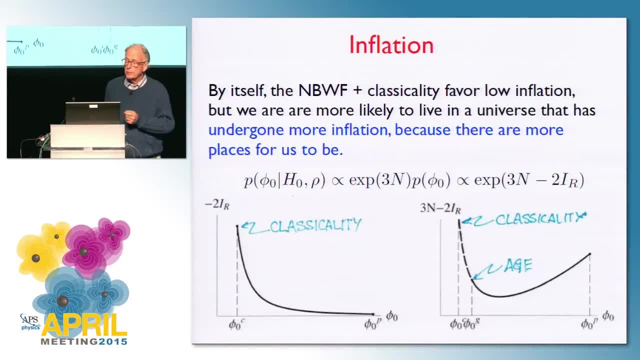 So the theory may predict probabilities for what occurs, but it's a different set of probabilities for what we would observe, because we're particular systems and we only have a probability to exist in any one Hubble volume. It's more probable that we exist in larger universes. 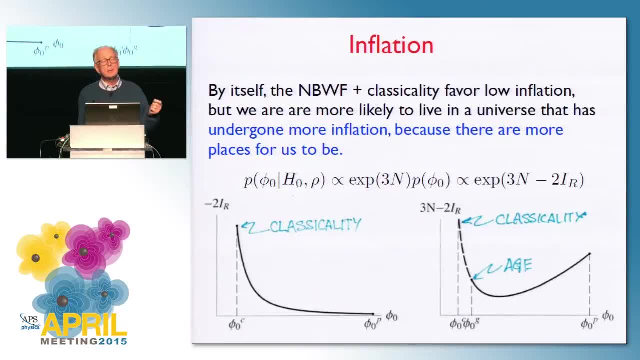 because there are more places for us to be predicted And that means that even though the probability for um inflation to occur- uh, with a large number of e-folds- is small, the probabilities for us to observe a lot of inflation by our observations is actually high. 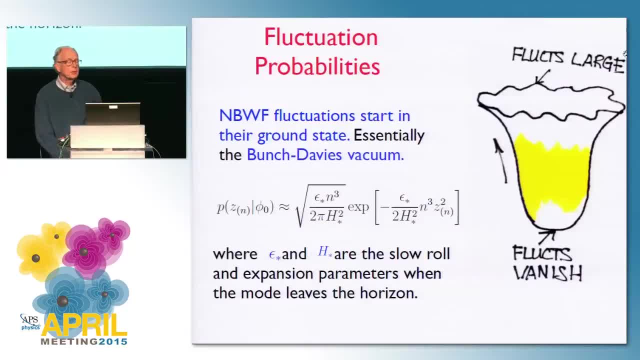 Thus the theory agrees with them. So let's look at the homogeneous and isotropic experiment. Uh well, that's homogeneous and isotropic. of course It's standard perturbation theory. to extend that by considering little fluctuations, right? 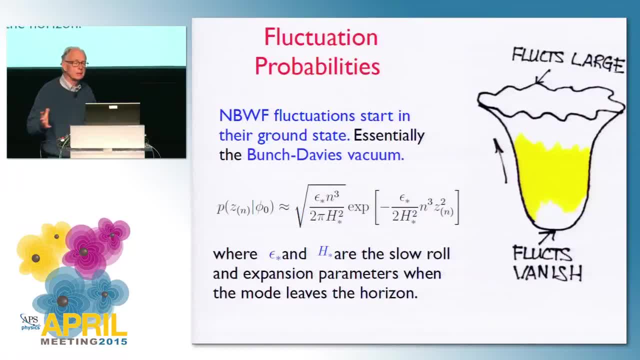 That's a typical graduate student problem. We did the homogeneous isotropic part. Now you can expand in fluctuations and uh calculate that, Since the no-boundary wave function is essentially a Euclidean construction, right? um, it won't surprise you. 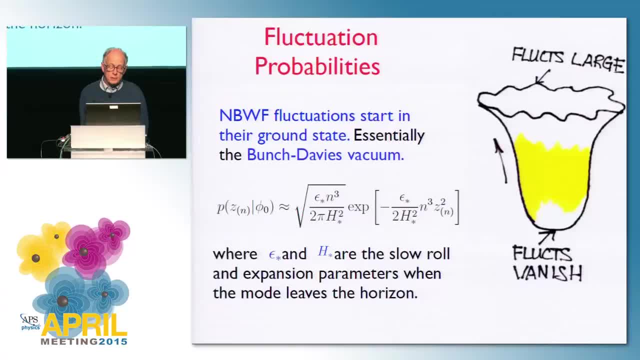 that the fluctuations in the ground state, something called the Bunch-Davis vacuum. uh, and if you know the technology of that, where these are the standard slow-roll parameters and these are the size of the fluctuations, uh, they give you the standard prediction. 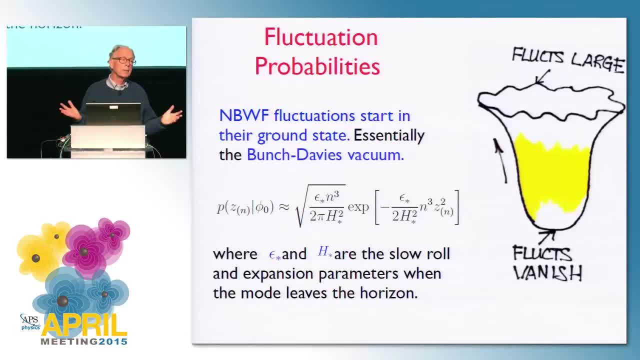 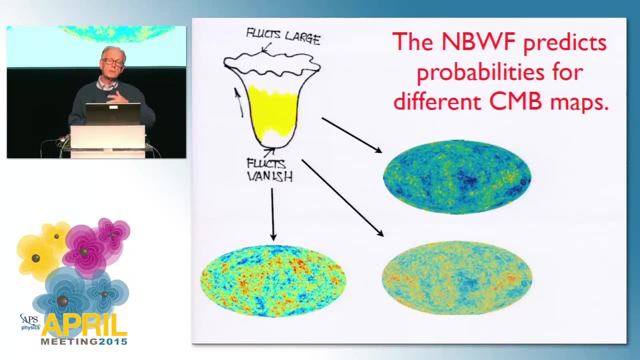 that's usually assumed in um in cosmology, to explain the scale-free invariant spectrum or something that we see, uh, in large scales. So this works pretty well also. In short, uh, the wave function predicts probabilities for different CMB maps. 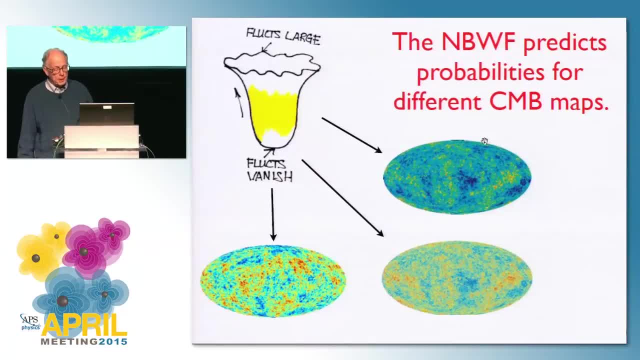 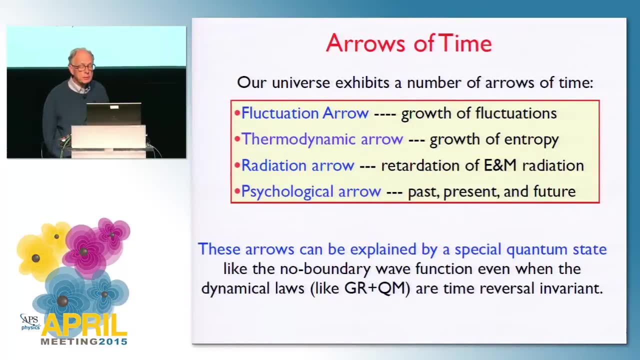 as we occurred, as we saw in the different- as in the preceding talk- Arrows of time. Well, our universe exhibits a number of arrows of time. So there's the fluctu- fluctuation arrow. The fluctuations seem to be small in the beginning. 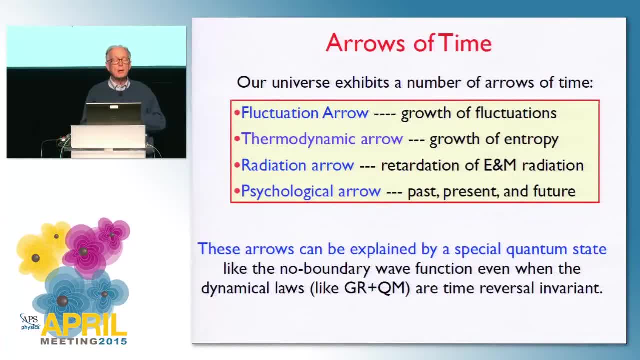 and grow as it goes on. There's the thermodynamic arrow, the growth of entropy right in the universe, The radiation arrow, uh, the retardation of electromagnetic ratio radiation, And the psychological arrow that we order prediction into past, present and future. 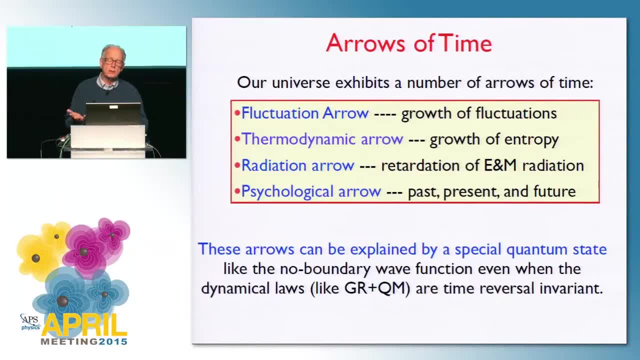 Uh, these arrows are all. I don't have time to go into it, but they're all essentially the same. They follow from the really from the fluctuation arrow And they can be explained by the special quantum state, like the no-boundary wave function. 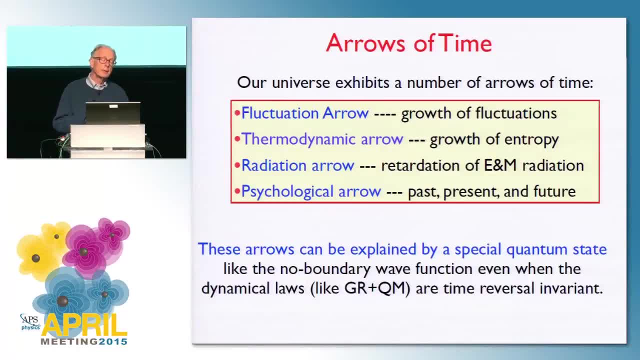 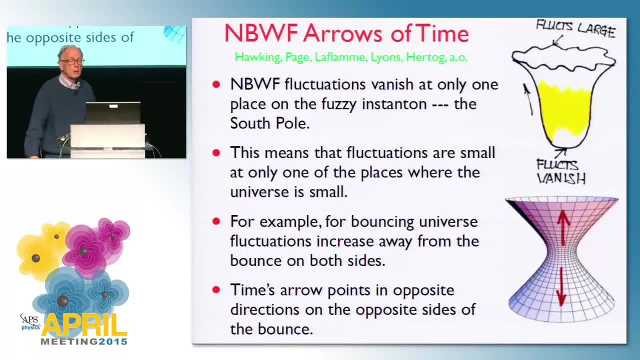 where the dynamical laws are time-symmetric right, but the um state of the uh fields is different in different uh geometries. So no-boundary wave functions vanish at one and only one place on the instanton. 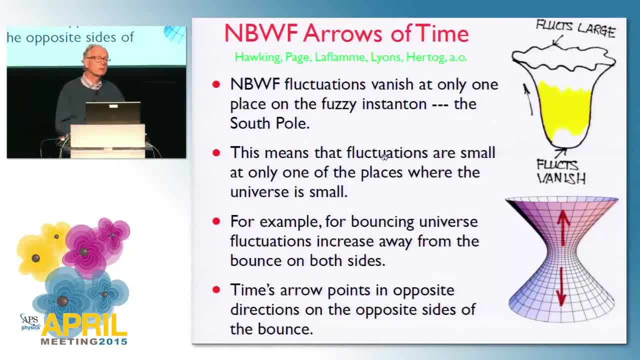 down here from symmetry. This means the fluxions turns out to mean the fluctuations are small and only at one place in the universe, uh, which is if we only have, um, uh, an expanding universe would be at the beginning. 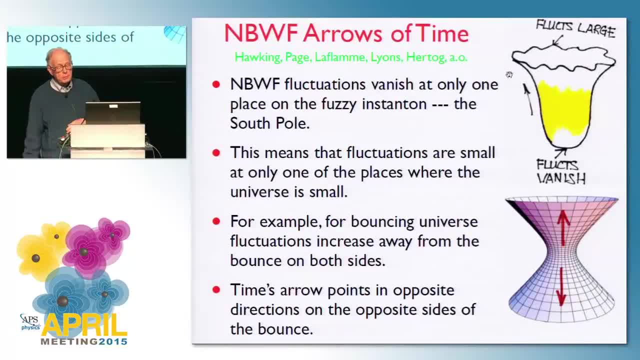 But an interesting example is what if we have a bouncing universe right that contracts and then re-expands, It turns out the fluctuations are not small at one end, large end, or the other, They're small in the middle. That means the arrow of times, all the arrows of time. 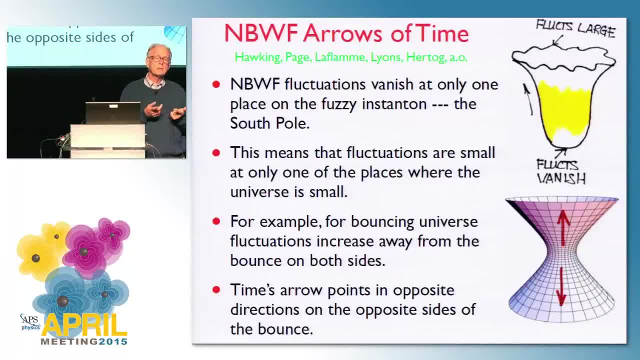 will point in opposite directions on opposite sides of the balance in a symmetric way. right, even though there's an arrow in each place. Uh, that's not very good for um getting observational uh information about the other side of the balance. 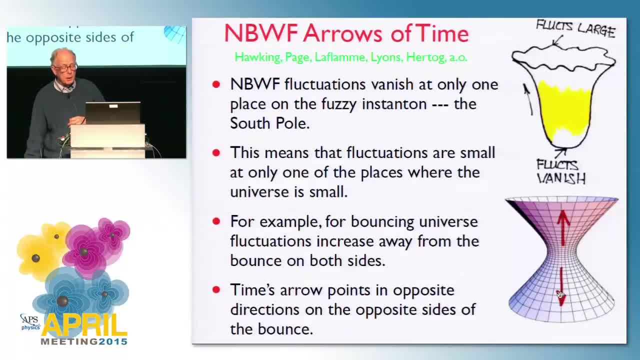 because uh people back here, uh will have had about as much chance of uh sending us information as we have sending information backward in time to um to uh tell people not to vote a certain way in an election. 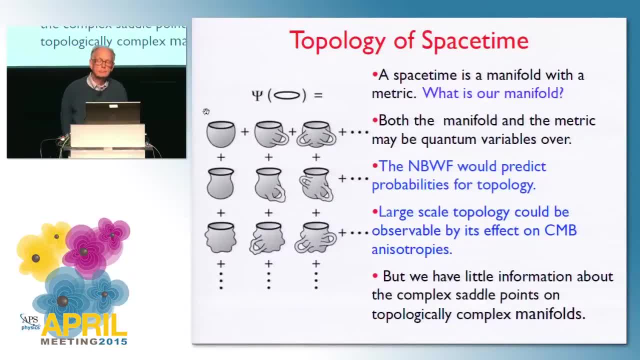 It's not gonna be uh done, Um well, I had a big list there, which I'll go over again. but there are some of the successes, but there are some things that are interesting, that, uh, we just haven't been able to do yet. 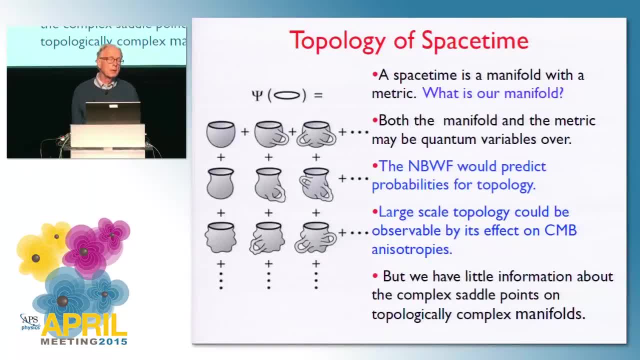 Uh, uh, space-time, uh, geometrically or mathematically, is a manifold with a metric on it. A manifold is just the topological structure of um, of of the geometry. So, for example, you can imagine, uh. 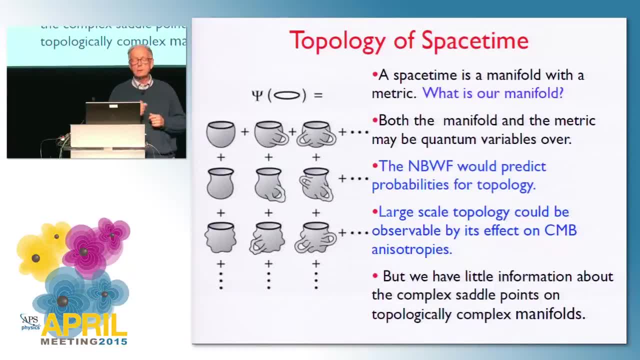 manifolds like a sphere, or have a handle on them, as in these fanciful pictures on the side, or like a, like a doughnut, and so forth. Uh, if we seek to uh to predict the classical metric, we might also seek to predict probabilities. 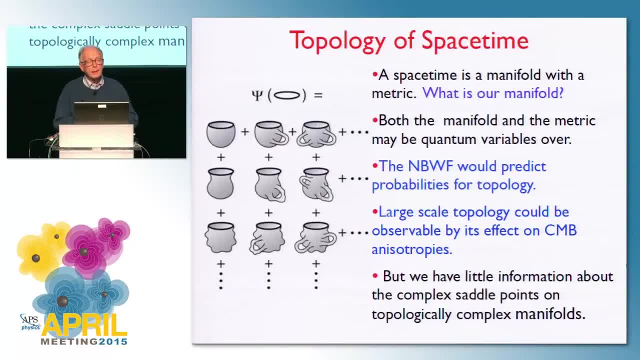 for what manifolds we have, And that has an observable effect if it's not on too large a scale. That is, imagine, for example, uh, the universe was like a torus or one of these halls of mirrors, you see, where you see infinite reflections going off. 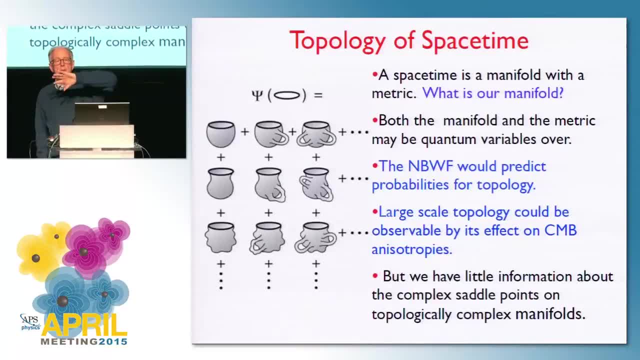 in different directions. That would have an effect on distorting the CMB that we observe, because you'd see one reflection of it, another reflection of it if it wasn't on too huge a scale, So large-scale topology at some level. 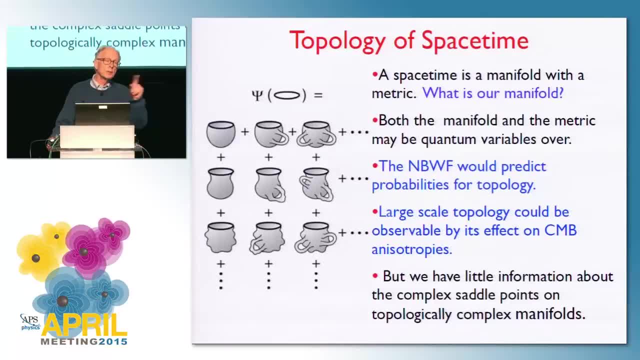 is detectable by its effects on the CMB and that's been looked for and so far there are no effects. But it's a very hard problem to do because I showed you how saddle points led to a very simple universe but we have very little information about. 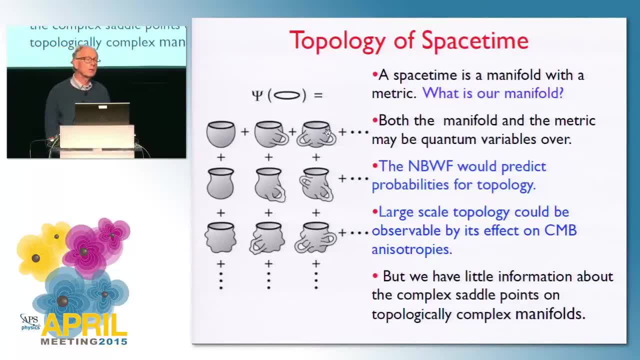 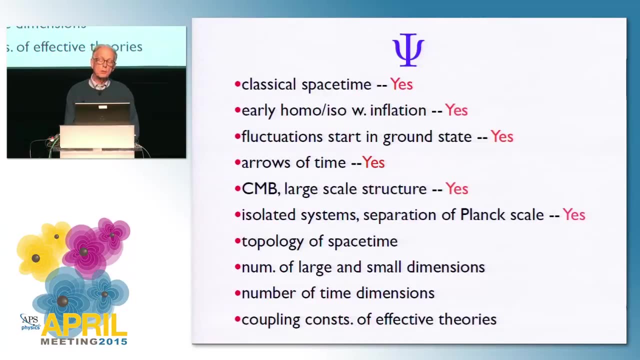 what kind of saddle points? complex saddle points would exist on manifolds with uh, complex, uh topology. But if we had them then we could actually um compute. So um, where are we on our scorecard? 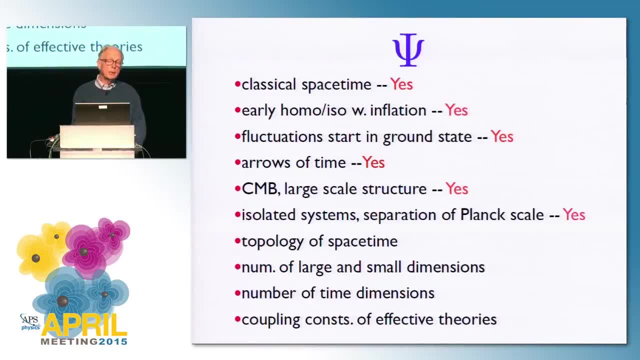 Uh, the features we might expect to be predicted, or here's the list I had in the beginning. Uh, classical spacetime: Yes, the theory does predict that the spacetime is classical and we're over what the classical spacetimes on very large scales are. 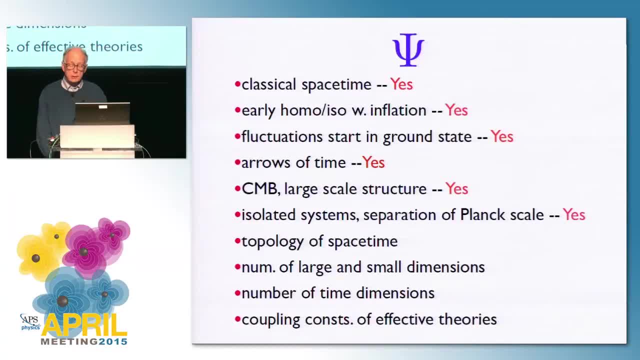 Early homogeneity and isotropy with inflation: Yes, it predicts that through the fluctuations, Fluctuations start in their ground state. Yes. Arrows of time: It certainly predicts the arrows of time as a special state in a time-symmetric theoretical framework. 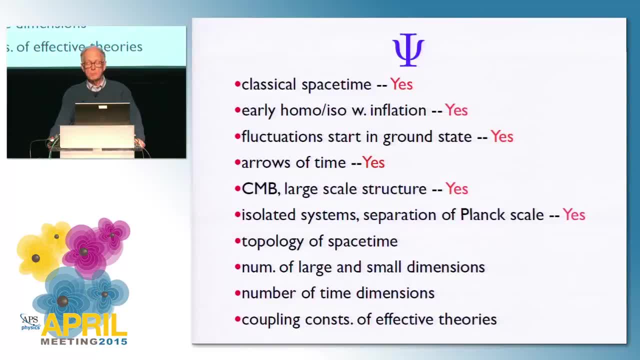 Uh, the CMB large-scale structure. Uh well, I There are a lot of things I didn't say here. Isolated systems, for example, The separation of the um- um of the Planck scale, The remarkable and very lucky fact. 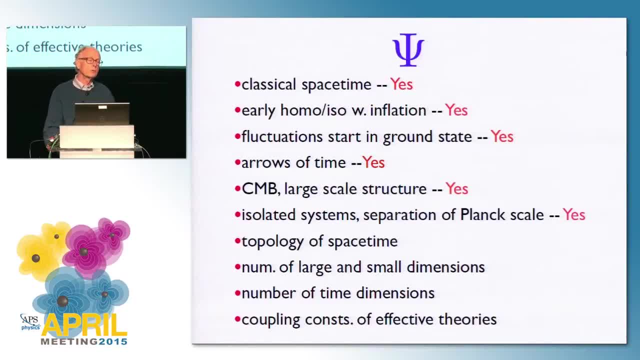 that we didn't have to know anything about quantum gravity to do the rest of physics right. We only had to um know about it in extreme circumstances: Topology of spacetime, number of large and small dimensions and principle predictor, et cetera. 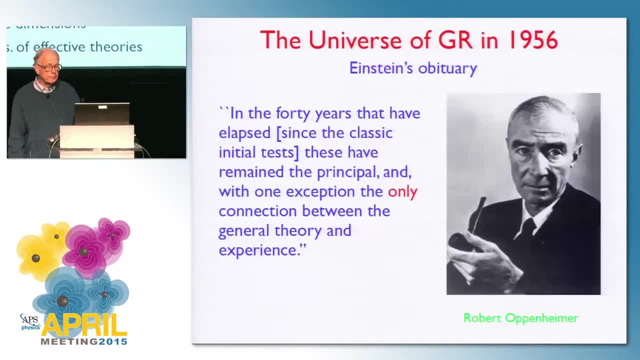 So some successes. I've only been able to report on a few. That's quantum cosmology, But in this centenary year it's maybe appropriate to think about um general relativity in a broader uh context, Um Robert Oppenheimer. 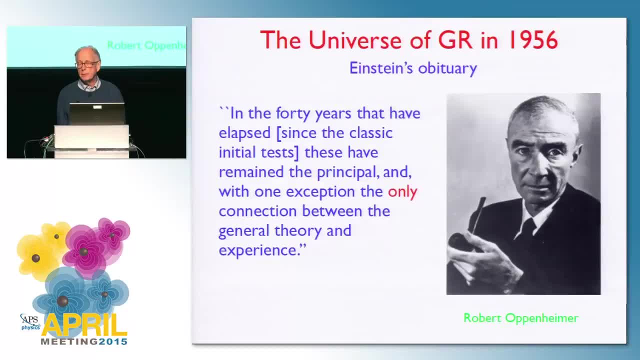 writing a eulogy in Reviews of Modern Physics, I think in 1956, right after um Einstein's death, was kind of critical of general relativity. He said, in the 40 years that have elapsed since the classic initial test, what he means. 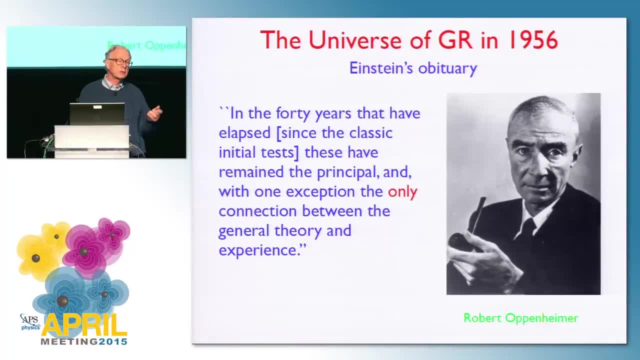 these have remained, Uh, the deflection of light, the perc-percession of the per- perihelion, the gravitational redshift, and so forth. Uh, these have remained the principle and with one exception: the only connection between general relativity and experience. 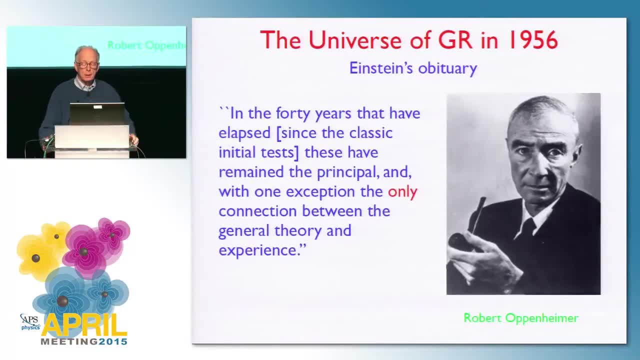 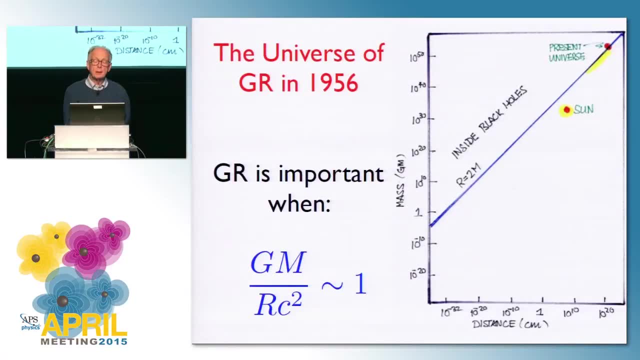 I think the implication is that the theory had been uh some in some sense of failure. And indeed, if you plot, um, make a plot, a convenient plot that I learned from Clifford Will, uh, uh, the mass of objects measured in grams going up this way. 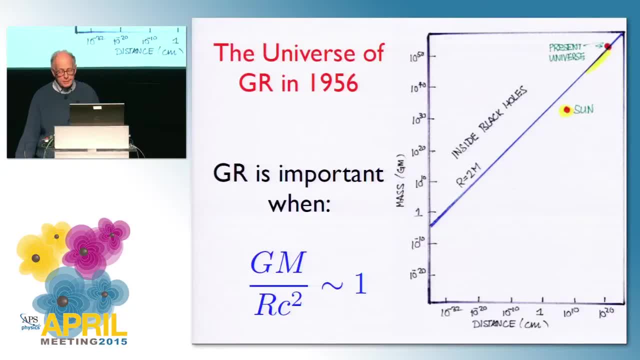 I apologize for the low quality of the um of the graphics here, uh, versus their size in uh centimeters. then, roughly speaking, relativity is important when the ratio gm over rc squared is approximately one, that is lying along this line here: 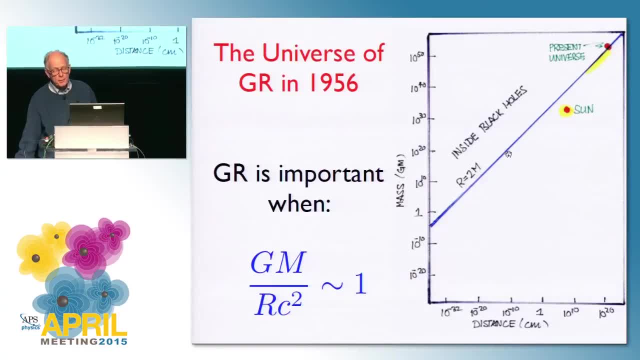 Can't be bigger than one because you're inside black holes. but the further phenomena, the closer to the line uh than um, the more relativistic effects are important. So the present universe, in some approximate way, um runs along this line from the Planck scale way down here. 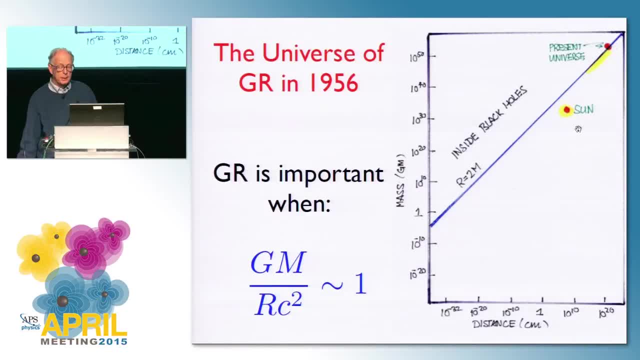 all the way up to the present. uh and the um, the sun. no, that's an order of 10 to the minus. fifth effect is somewhat close to the line and that's the way it looked in 1956.. 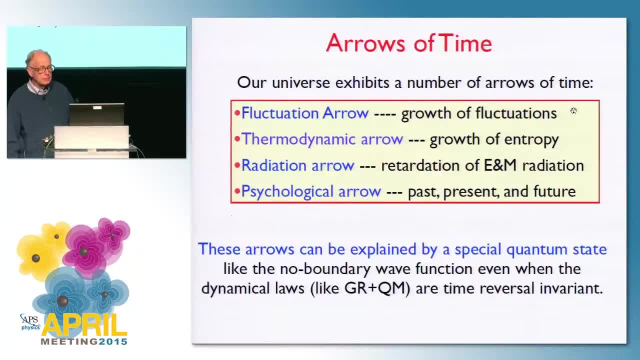 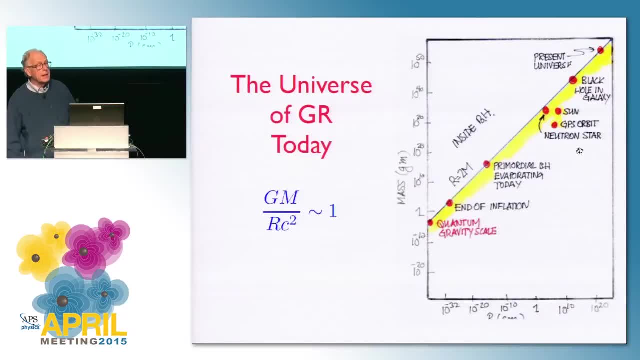 Oops, Ah yeah, Today it looks better. astrophysically There are a lot of things. There's the quantum gravity scale down here, the end of inflation. so you know, we have pretty good evidence for some sort of inflation occurring. 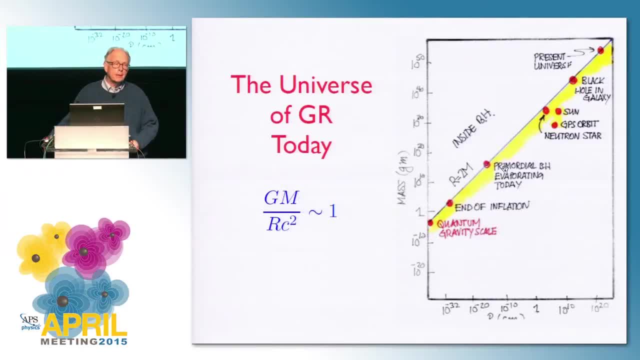 Uh, primordial black hole evaporating today, which we haven't seen yet in the, in the diffuse x-ray background. Uh, and many more tests of the, the theory of relativity on solar system scales remarkably accurate, one, for example: 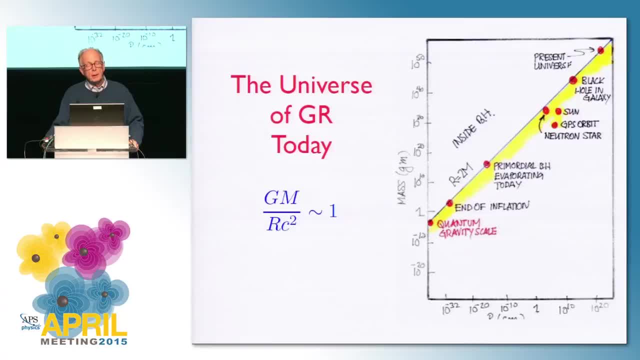 the test of the bending of, or the Shapiro time delay uh by the Cassini mission to a part in 10 to the fifth. That was unheard of, certainly Uh. neutron stars, properties of neutron stars, maximum masses and so forth. 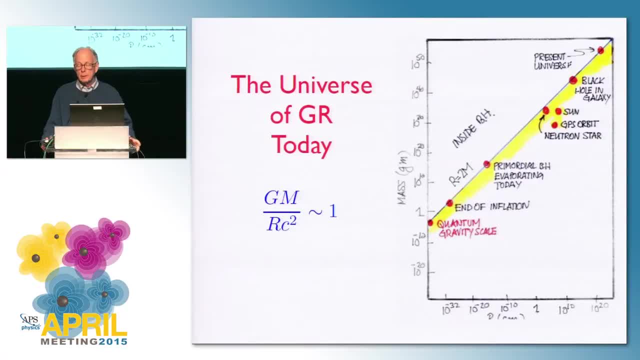 Uh and um uh. the global positioning system, as Cliff stressed for you the other day, would fail in a half an hour if it didn't compensate for the effects of the solar system, The effects of general relativity, Black holes in galaxies- we we uh have. 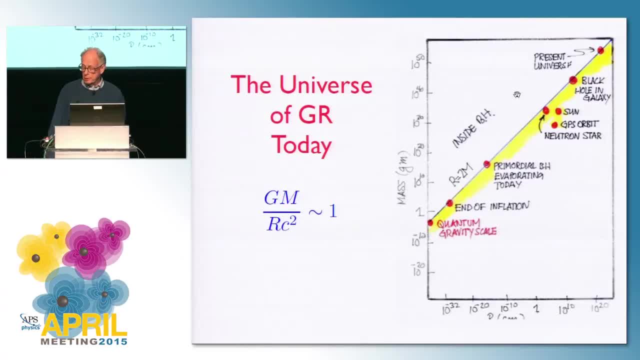 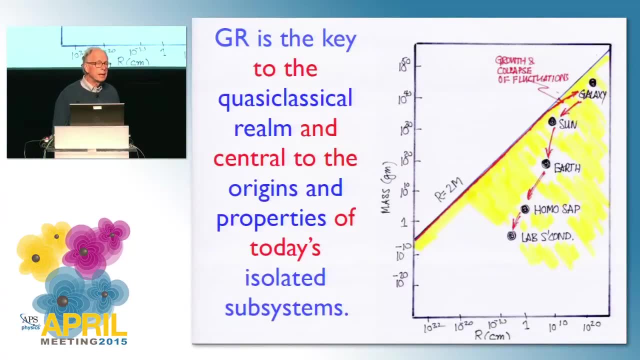 and, of course, there's a present universe, So it's much better today. But if you're interested not in just what's going on today, but what, when, where did all this stuff come from? right, then GR, first of all, is the key, as I've already mentioned. 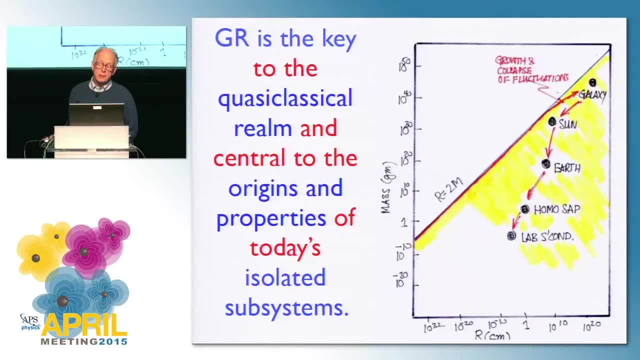 to the existence of the quasi-classical realm, to the utility of classical physics, and it's central to the origin and properties of today's isolated systems. So if you're working in a laboratory and you trace back right where we are, 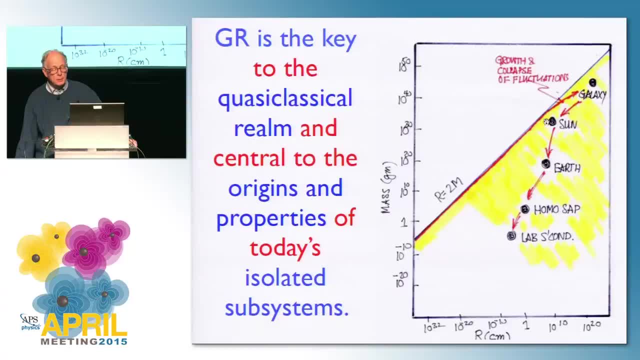 you're talking about a curve that started out here from the Planck scale came up, then the fluctuations grew under the action of gravitational. the quantum fluctuations grew under the action of gravitational attraction- uh to collapse, uh, eventually to make galaxies. 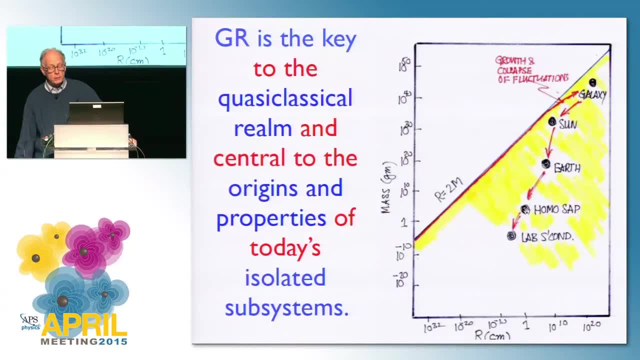 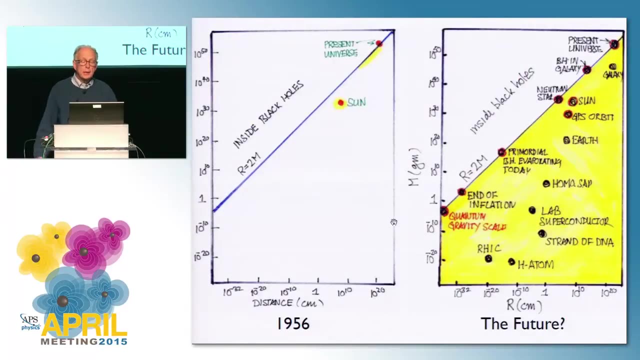 stars, planets, very small fluctuations, us and doing experiments in laboratories. So if you're interested at all in history, you're interested in general relativity, both classical and quantum. So in 1956, it looked like this: 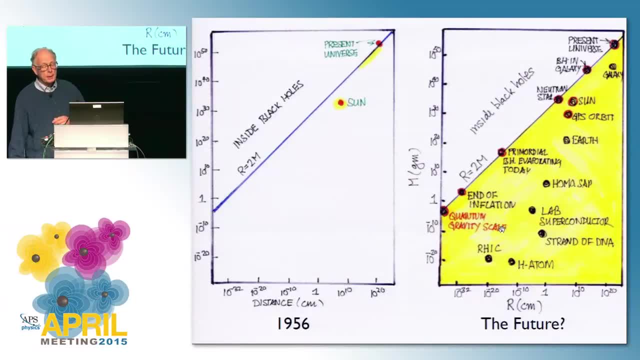 But in the future, uh, it may, um, it may be look more like this: There's increasing evidence that gravity might be in some sense, a theory of everything right, where everything is uh effective And uh it's uh expected by general relativity. 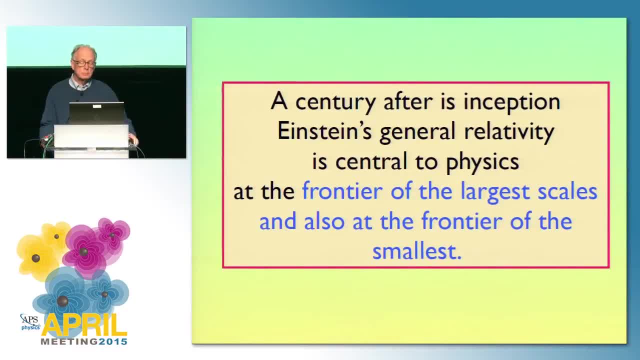 going backward, So a century after its inception. Einstein's general relativity is central uh to physics, both on the frontier of the very large and also the frontiers of the very small. Um Martin Seligman, who was president. 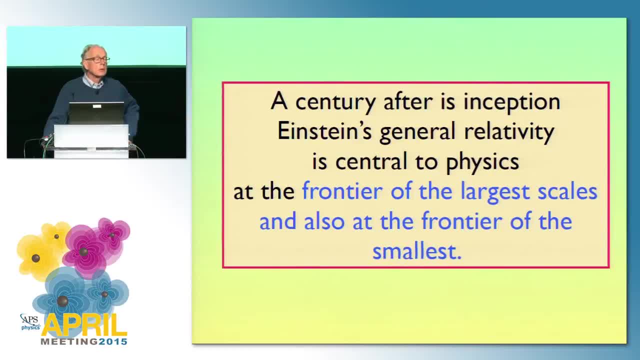 of the American Psychiatric Association was, uh, the subject of a CNN, CNN, um, uh, special. and they said to him: well, what we're interested in is the state of American psychiatry today. So but we had to be short. 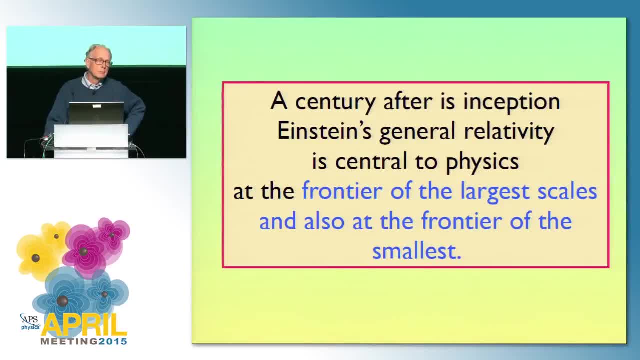 How would you summarize that? in one word: And he said good, And then they said well. uh, that's not very informative. How about two words? And he said not good And they said well. you just contradicted yourself. 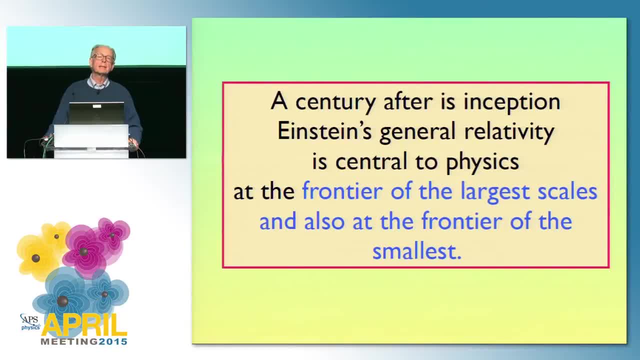 So how about three words? And he said: not good enough. And, ladies and gentlemen, if I had to summarize for you in one word, two words, three words and four words, the state of quantum gravity and quantum cosmology today, 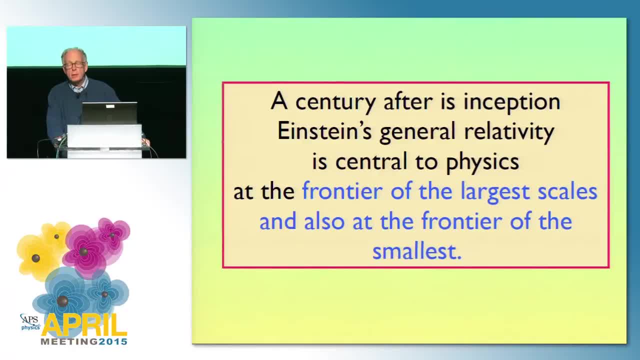 it would be exactly that. It's good, Amazing progress has been made. A lot of stuff- questions- that we never asked before- have been addressed, uh, and are keeping on being addressed. It's not good, right, Because we're quite far from any having definitive resolution. 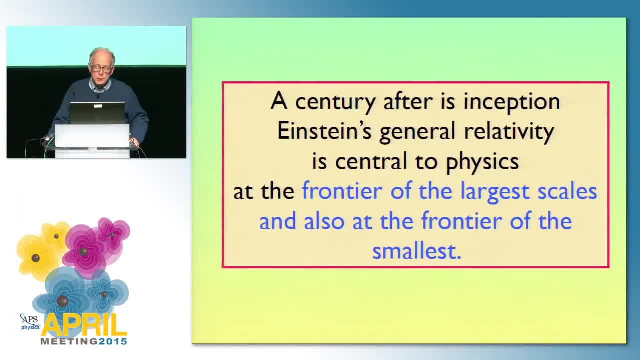 There are a lot of puzzles, like black hole evaporation, that are confusing. In short, uh, it's good, but it's not yet good enough. Thank you, You mentioned that black energy was tan to the exponent uh 28 electron volts. 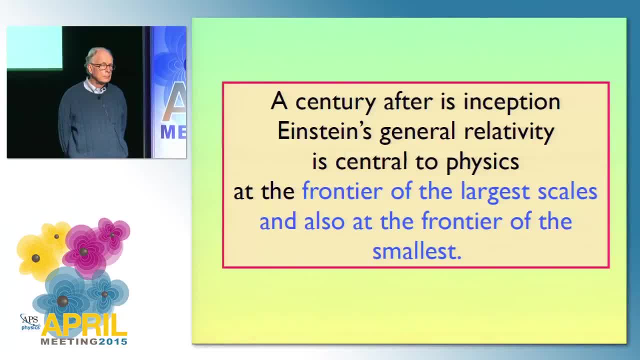 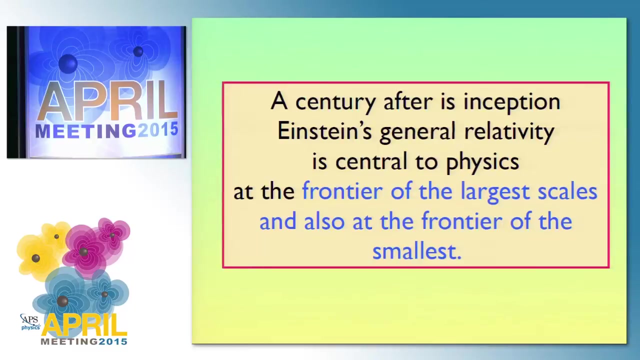 And yet the donut-shaped singularity that generated the Big Bang that had an energy of 10 to the exponent 90 electron volts. Does that mean that quantum mechanics is invalid in those regions? Because the energy of the Big Bang is 10 to the exponent 60 times greater? 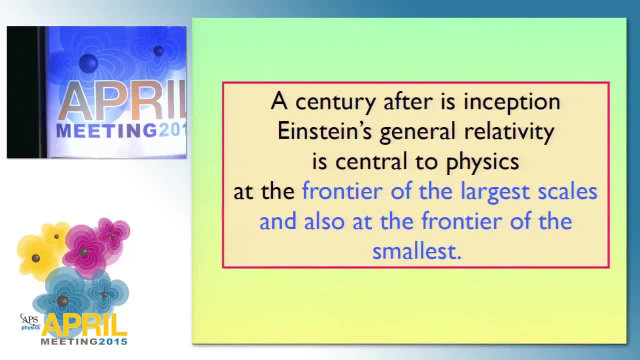 than the largest energy of that Planck cube. If I had more time. oh, I agree with your question, right? How do we know quantum mechanics applies to the universe as a whole? No, we don't. Uh, the biggest laboratory experiments, like, uh, Friedman et al. 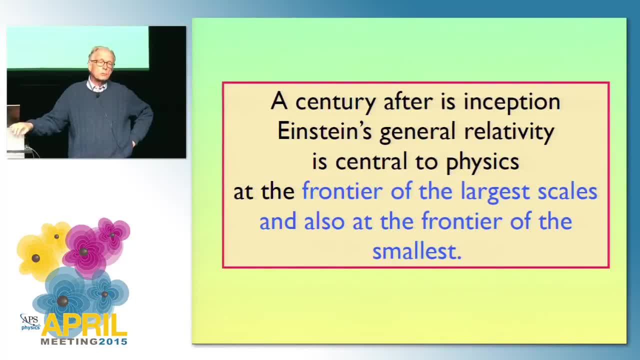 on Josephson junctions, uh, you know, only go up to um 10 to the 8th. well, there's some dispute in condensed matter, physics, uh particles. So we only had the theories only tested on um, on, uh laboratory scales. 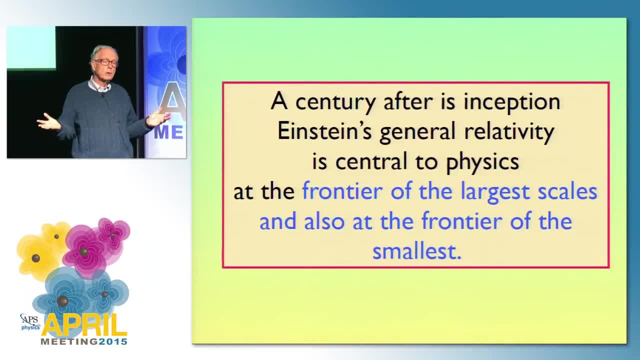 What's the justification for extrapolating it to these very large scales? First of all, it seems to work, for example, on the story about the quantum fluctuations generating large-scale structure, But frankly, we'll only find out whether it applies if we do it. 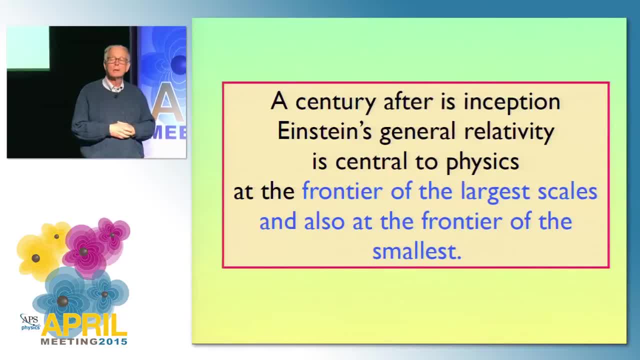 and then see if there's some horizon. All right, Thank you. Question over here: I wonder if there's some anthropomorphic hypothesis in your work. Anthropomorphic, You said that, uh, inflation could have happened because there's more space for us. 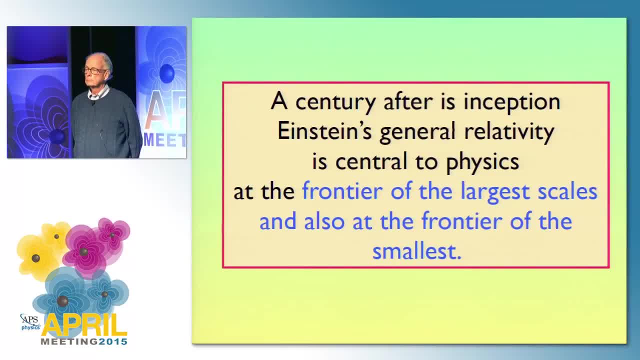 So in your model, does that mean that, uh, is it necessary or sufficient for there to be inflation, for there to be people? I don't think we know anything like necessary and sufficient because, uh, we only have one universe to study. 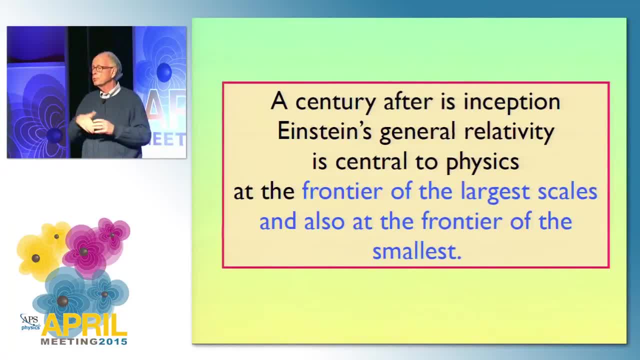 But you're right, Anthropic reasoning, so-called that people did a long time ago, is automatic in quantum uh, quantum cosmology, because all of our uh observations are contingent, as Bohr said right on a description of the observational situation. 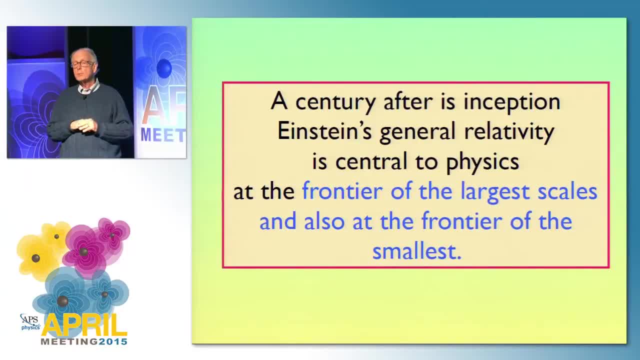 For example, it doesn't make any sense to say, uh, what do you predict for the temperature of the microwave background, Because it varies in time and it depends on uh what, uh what time it is. So you have to put that kind of information. 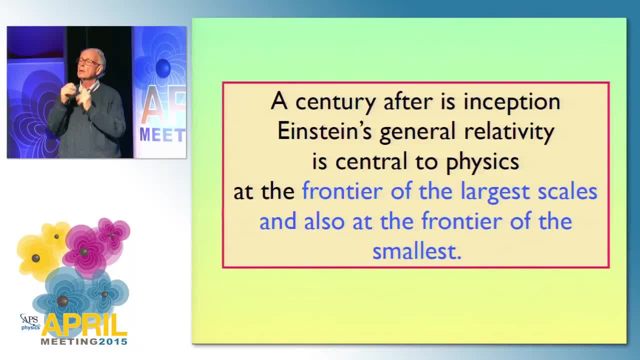 and description of the observational situation in including us. So that means that we won't observe what is where we cannot exist. So in uh imagine, as in contemporary landscape theories, the cosmological constant varies from place to place in the universe. 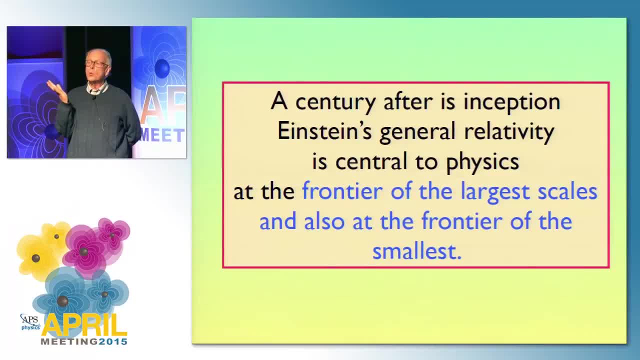 uh, and its typical value is uh of order one in Planck units, not 10 to the minus 122 as it is in uh. in our case, Uh, we wouldn't observe one because a large cosmological constant, as Weinberg, Barrow and Tipler and other people showed, 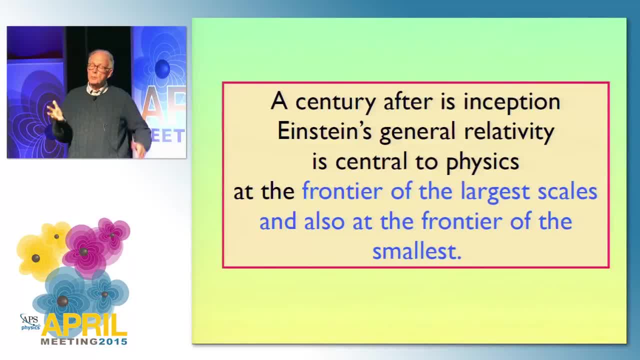 that's much, uh little. only a little bit larger would mean the universe would expand so rapidly the galaxies wouldn't form. So if you calculate the, the probabilities for what occurs, it might be very large, but the probability of what we will see is very small. 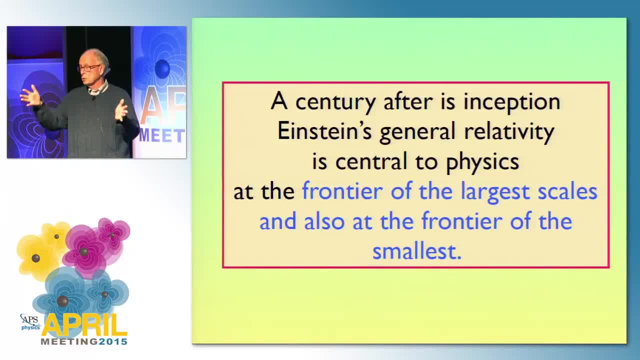 And those calculations give you a number which is, you know, with plenty of assumptions, give you, give you a number which is essentially, um, the largest it could be and still be consistent with galaxy formation by um, uh, by 13 giga years.